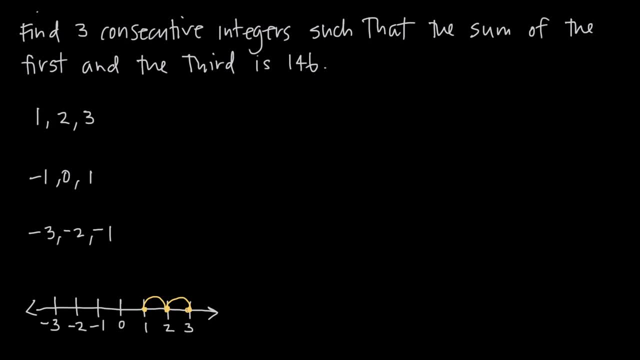 And because we can connect them like this: we know they're consecutive Negative 1,, 0, and 1, we have negative 1,, we have 0, and we have positive 1.. We can connect those three. We also have here negative 3,, negative 2, and negative 1.. Because we can connect those: 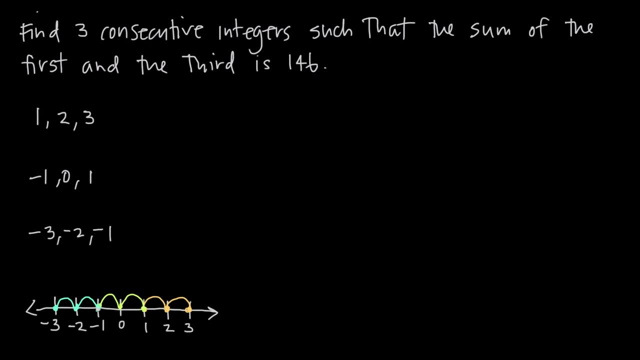 without lifting up our pencil. we know that those are consecutive integers also. So now we have this problem where we need to find three consecutive integers. So we need to find three consecutive integers. So we need to find three consecutive integers such that the sum of the first and the third integer is 146.. Well, we can do this by calling. 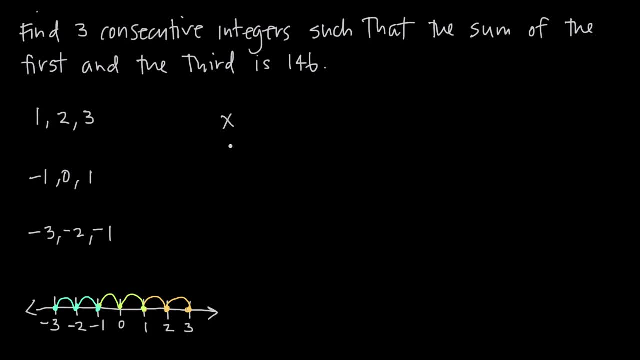 our first integer x, And if our integers are consecutive, then our second integer is going to be x plus 1.. Our third integer is going to be x plus 2.. Now, this should make sense to us. We can always test ourselves, because if we pretend that our first integer is 1,, 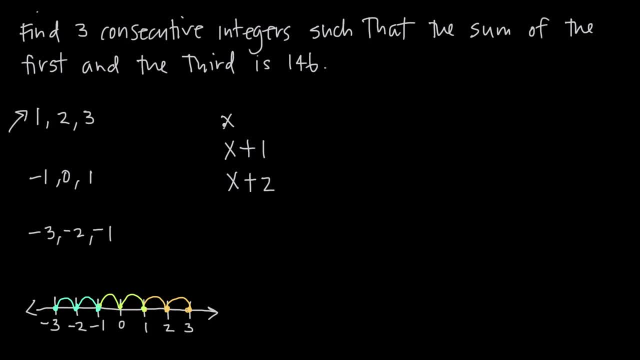 as in this consecutive integer series here, if we say our first integer is 1, then we're going to plug in 1 for x and see what we get. So plugging in 1 for x, here we're going to get 1.. Plugging 1 in for x: here we get 1 plus 1 is 2.. And plugging 1 in for x: here: 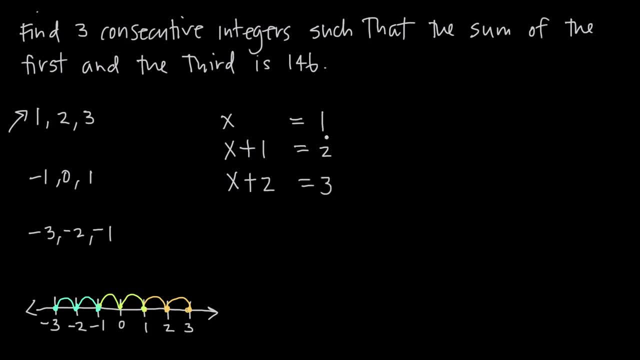 we get: 1 plus 2 is equal to 3.. And we can see here that we get three consecutive integers: 1, 2, and 3.. So we're representing these consecutive integers as x, x plus 1, and x plus 2.. So 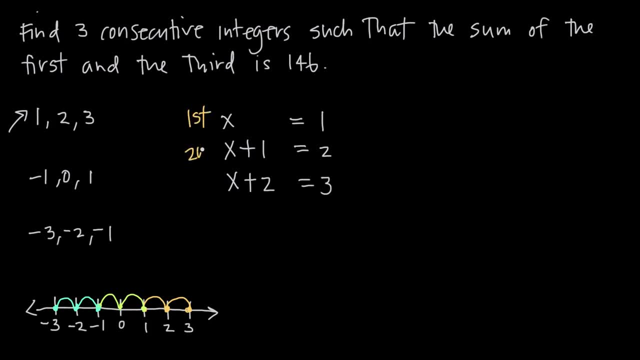 our first one here. this is our first integer, our second integer and our third integer. What this problem is asking us to do is add the first and the third together and get 146.. The first and the third, which means add them together. we have our first integer x and 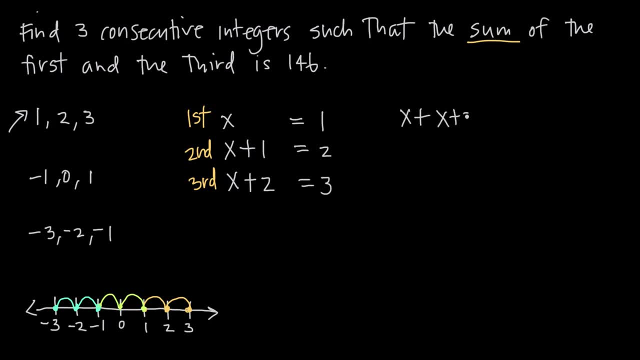 our third integer: x plus 2, so plus x plus 2.. And we want to know when this is equal to 146. Remember, is always means equal, So equal to 146. And now we just need to solve this equation for x. So x plus x is 2x plus 2 is equal to 146.. If we subtract 2 from both. 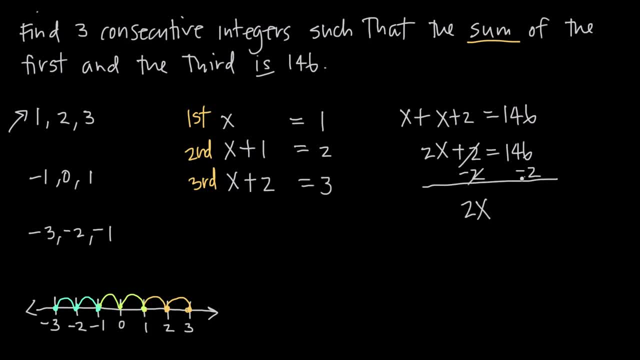 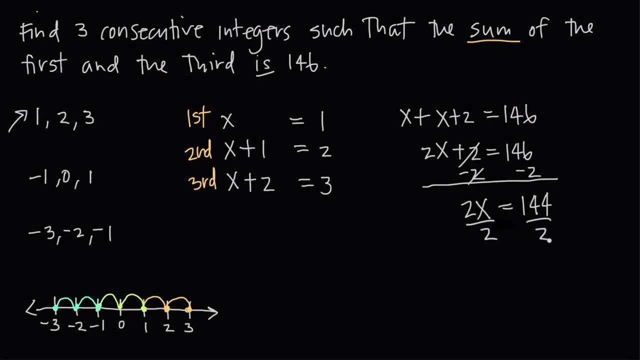 sides we get: 146 plus 2 is equal to 146.. So 146 plus 2 is equal to 146.. So 146 plus 2 is equal to 2x. And then 146 minus 2 on the right-hand side gives us 144.. Dividing: